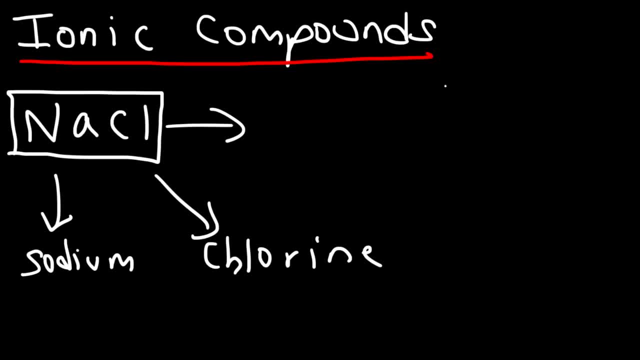 ionic compound. Ionic compounds are those that are composed of ions. we have the sodium ion and the chloride ion. a positively charged ion is known as a cation and a negatively charged ion is known as an anion. now, keep in mind the way you name the anion, is you change the ending from INE to IDE, and so this: 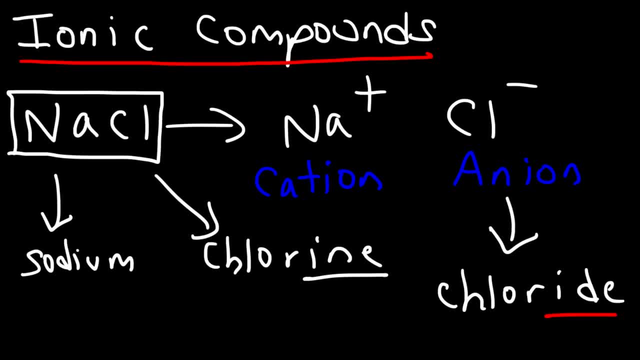 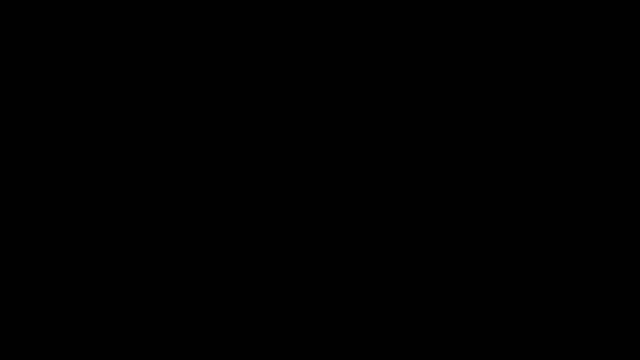 is important. you want to make sure you take note of this fact. when naming an anion, you need to add the suffix IDE. so to name NaCl, it's called sodium chloride. now let's try another example: MgBr2. so what do you think we need to do in? 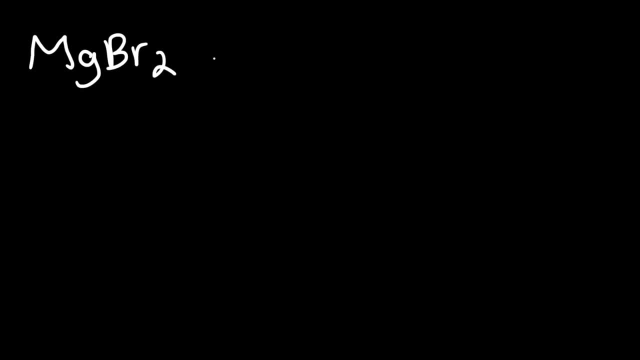 order to name this particular ionic compound. if you want to try it, go ahead. so the first thing you need to do is name the first element. so what is the name for Mg? if you use a periodic table, this is called magnesium. now, the second element, Br, stands for bromine. however, we need to replace. well, let's 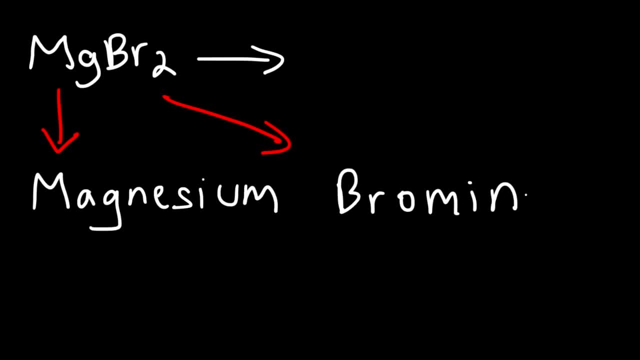 write it first. now, instead of writing bromine, we need to replace the last three letters with IDE. so this is going to be bromide and that's how you can name MgBr2. it's called magnesium bromide. so remember, when naming ionic compounds, you simply. 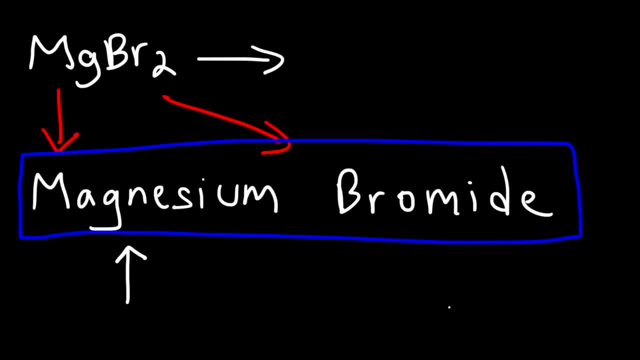 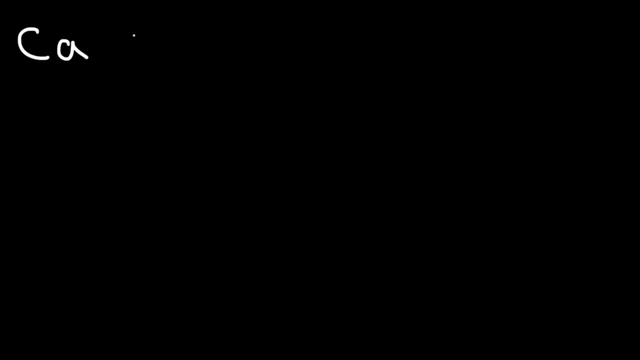 need to write the name of the first element, but for the second one, make sure to add the suffix IDE. now let's try some other examples. let's name these two. I got it: compounds- see a o&alp. so what do you think the names are for these two? mum to see a stands for. 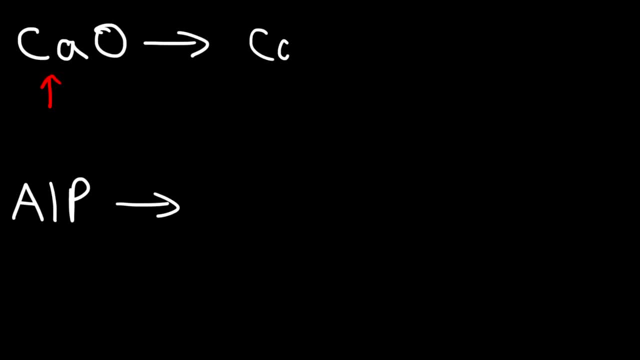 what element see? a is called calcium, educ oxygen. however, the last three letters has to be an I backwards, so you take care of your… be IDE. So instead of writing oxygen, we're going to write oxide, And so that's how you can name that particular ionic compound. Now what about the next one, ALP? AL stands for aluminum. 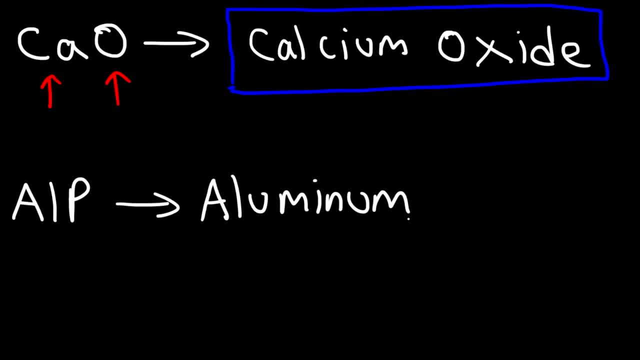 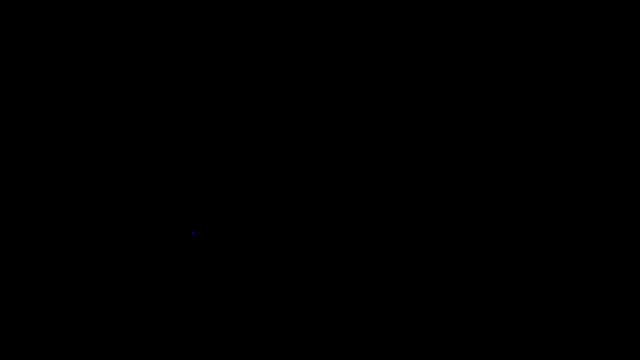 and P is phosphorus, but it's going to be called phosphide. So this is aluminum phosphide. So it's not very difficult to name ionic compounds. but there are some more challenging examples. You need to be familiar with certain polyatomic ions. Now I'm not going to go over. 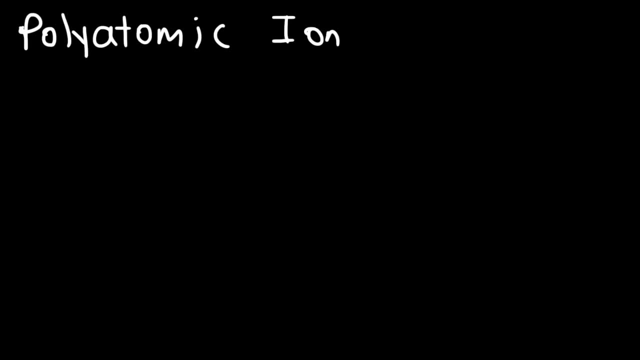 all of them, but just a few. So, for instance, you need to know that NO3- this is called nitrate, NO2- with one less oxygen, this is called nitrite, And you'll see this pattern often ATE has one. 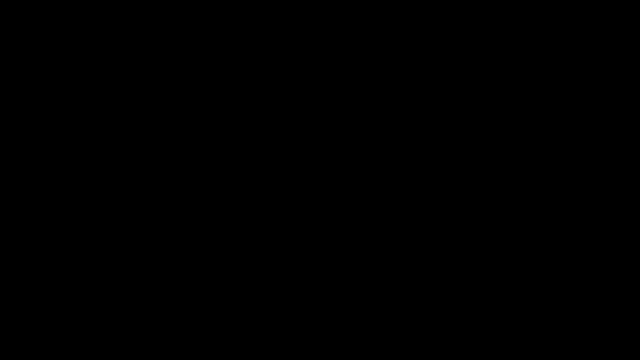 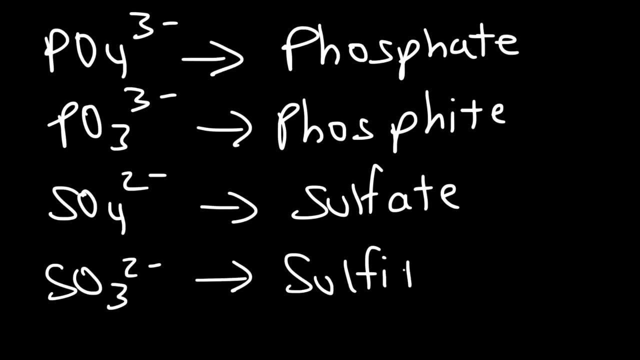 more oxygen than ITE. Some other polyatomic ions you want to be familiar with is: PO43- this is known as phosphate- You may want to write these down, by the way. PO3- this is known as SO4- This is called sulfate And SO3- is known as sulfite. Now, some other ones that you. 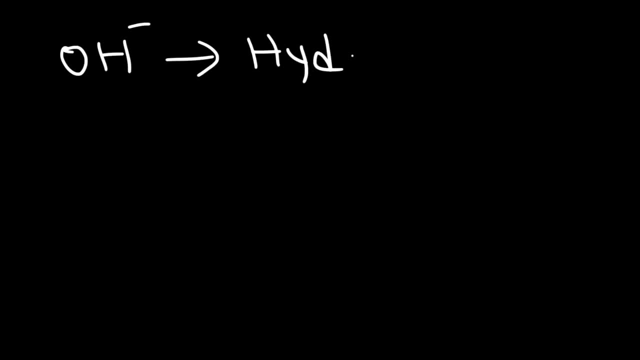 want to be familiar with is OH-. this is called hydroxide. And then you have CN- that's known as cyanide CR04- which is known as cyanide CR04- which is known as cyanide 2-. this is called chromate, and if you see CR 207 2- that's called dichromate. 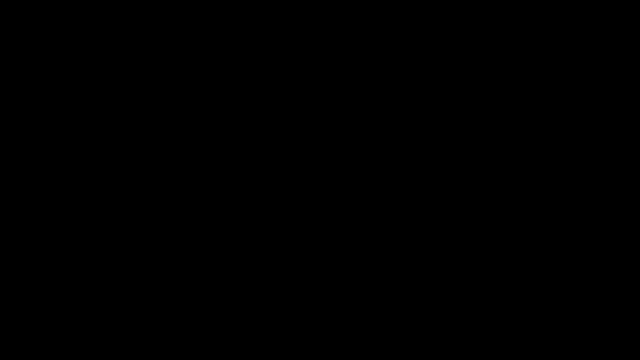 now there are some other ones, but let's stick with that. so, based on the list that you saw previously, how can we use that list to name the following compounds? so first we need to look at the first element, K, using the periodic table. K stands for potassium, so that is the K plus ion. the second one is a. 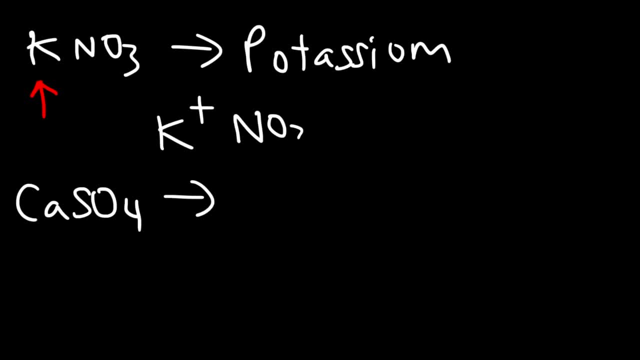 polyatomic ion. it's the NO3 minus ion which is called nitrate, and so this is how you name it. so this is how you name it. so this is how you name it. so this is how we name KNO3: it's simply potassium nitrate. now for the next one. we have CA. 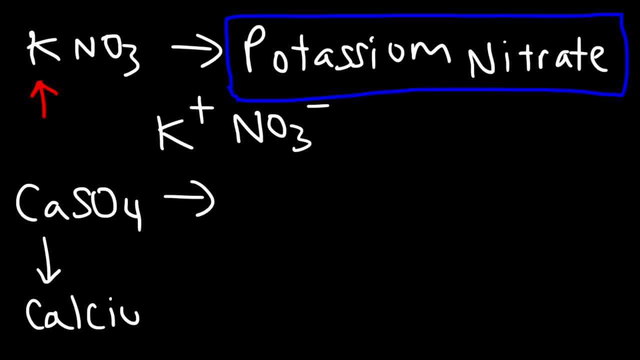 which stands for calcium and SO4, is called sulfate. so combined this is calcium sulfate, and so it's very straightforward to name ionic compounds with polyatomic ions. it's not that difficult. you have to remember that. you have to remember that. you have to remember that you have to. 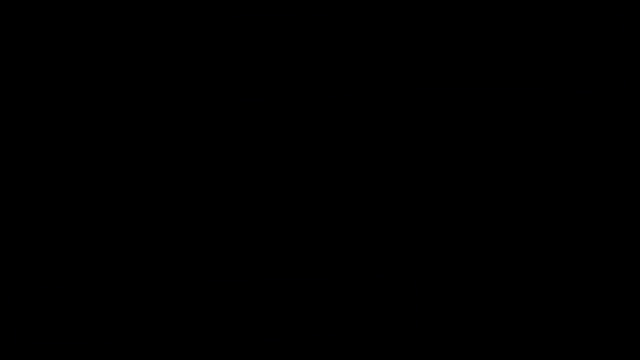 memorize the polyatomic ions. there's no other way around it. now, the next example that we are going to go over involves transition metals, so let's try these two examples. the first one is FeCl2 and the second one FeCl3. now how would you name these two compounds? looking at the first one, Fe is called. 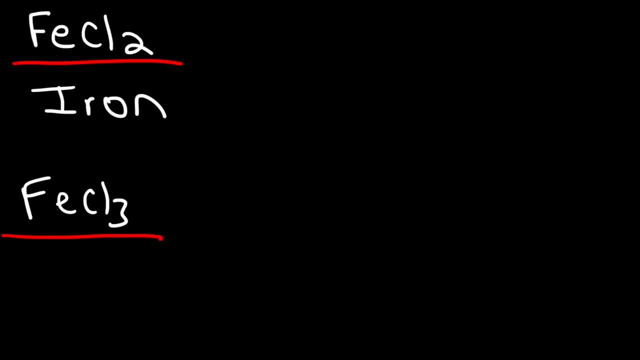 iron and Cl is called iron. so these two compounds are called iron and Cl is chlorine. but for an ionic compound we're going to use the word chloride. well, we can apply the same thing to FeCl3: it also would be called iron chloride. however, we can't apply the same name to two different compounds, so we need. 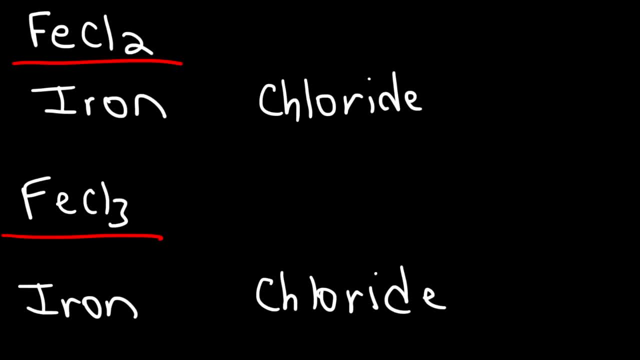 something else. we need something more. it turns out that FeCl2 is called iron 2 chloride and FeCl3 is iron 3 chloride, and the reason for that is the FeCl2 compound contains the Fe2 plus ion, whereas FeCl3 it contains the Fe3 plus ion. and so when dealing with certain 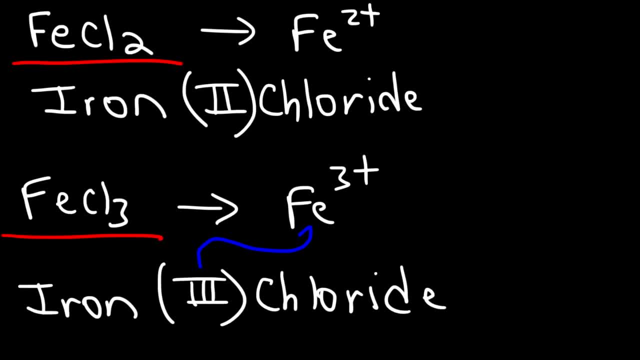 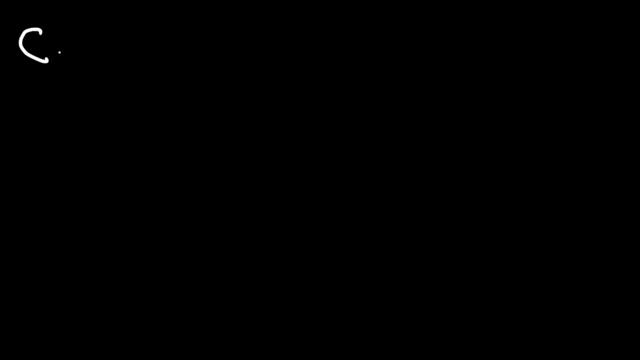 transition metals, you need to use the roman numeral to indicate the charge or the oxidation state of the ion. now let's try this one: CuS. how can we name this particular ionic compound? well, we know that Cu stands for copper, S is sulfur, but we need the end in ide, so copper sulfide. but now is it. 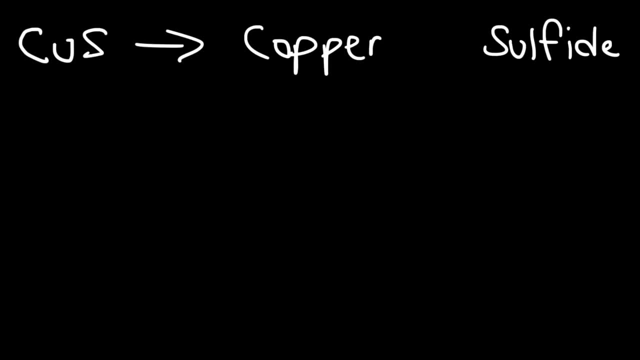 copper 1- sulfide. copper 2- sulfide. copper 3- sulfide. which one is it? well, we need to determine the charge on the copper atom, or rather the copper ion, and so first we need to chart, excuse me, determine the charge on the sulfur anion. now, sulfur is a chalcogen found in group 6a of the 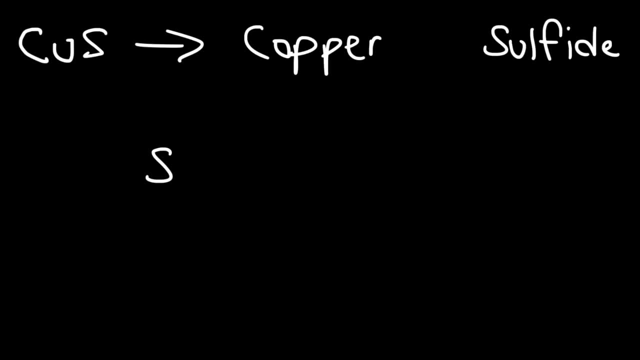 periodic table and those elements. they form negative 2 charged anions. now copper has to have the same charge in order to balance the charges of the compound. so copper has to be 2 plus and you can write an equation to find the answer if you write Cu plus anion. 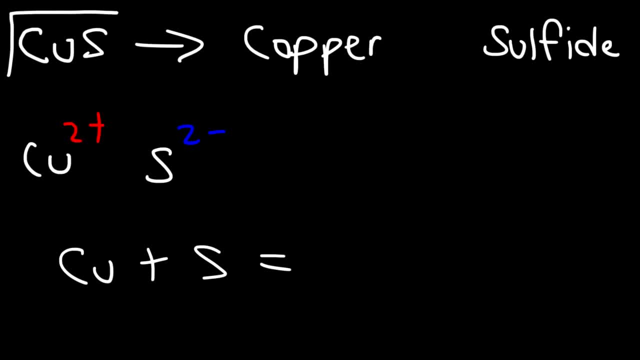 S and notice that the net charge of this entire compound is 0. so you set it equal to 0, and we know that sulfur has a minus 2 charge. so, solving for copper, we need to add 2 to both sides, so thus copper has a 2 plus charge, and so we're. 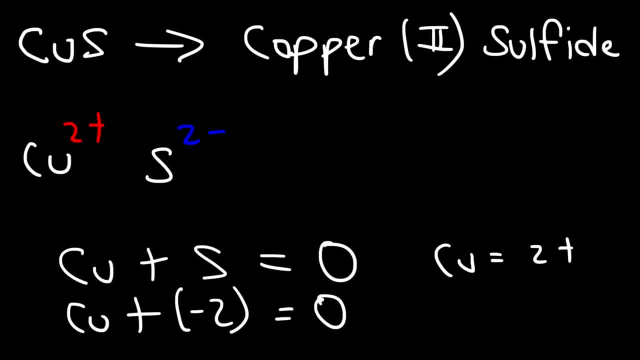 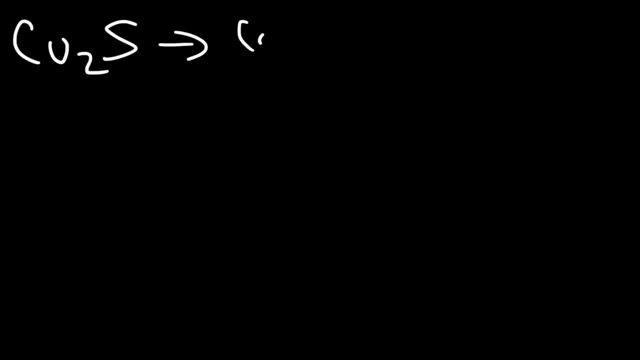 going to call it copper 2 sulfide. now let me give you another example. let's name this one Cu2S. so we know it's going to be copper sulfide, but the oxidation state is different. so let's write an equation. this time we have two copper atoms: one. 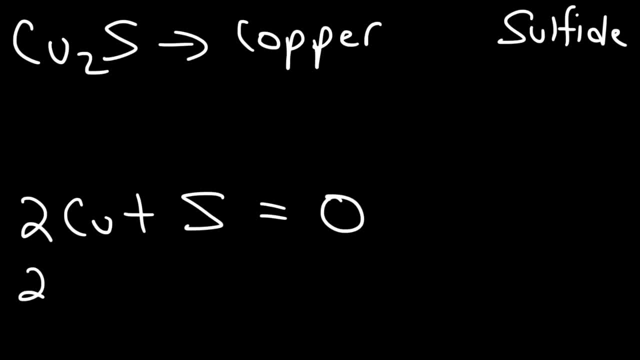 sulfur atom and the net charge has to add up to 0. so since we're solving for copper, let's replace it with an X. sulfur has a minus 2 charge. so if we add 2 to both sides of the equation we'll get: 2x is equal to 2.